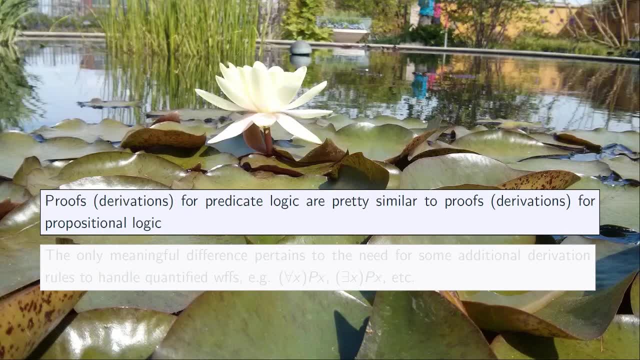 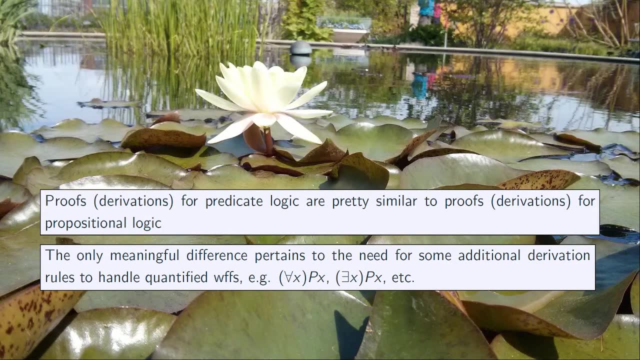 on propositional logic proofs because there is a lot of carryover. The significant or meaningful difference pertains to the need for some additional derivation rules to handle quantified, well-formed formulas, That is, in predicate logic proofs we have formulas where the main operator is 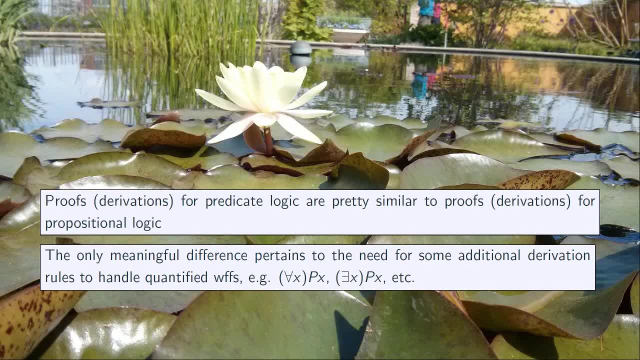 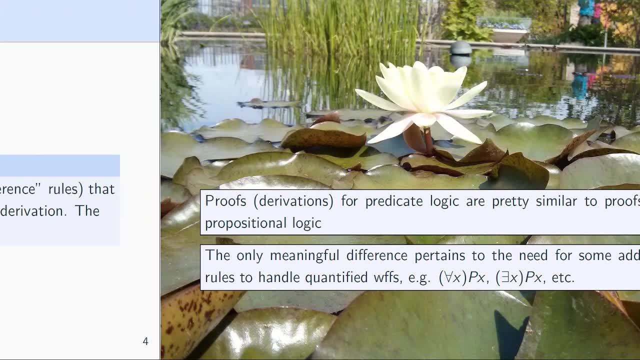 the universal quantifier or the existential quantifier, and we'll introduce some derivation rules that allow us to reason with or to these types of well-formed formulas. In this video, what I like to do is just to go over some terms that are important for understanding what's going on. 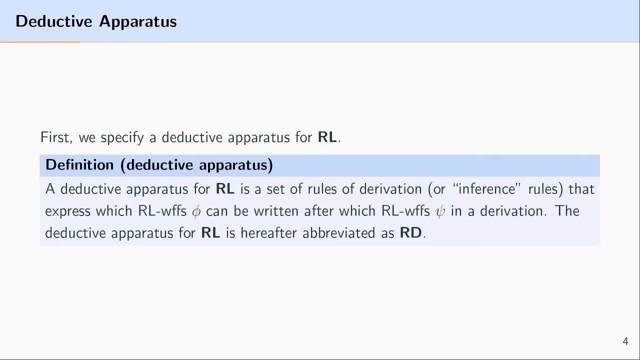 when we talk about predicate logic proofs. The first part is the deductive apparatus for predicate logic. The deductive apparatus for predicate logic refers to a set of rules of derivation. These are rules that express which well-formed formulas can be written, after which well-formed 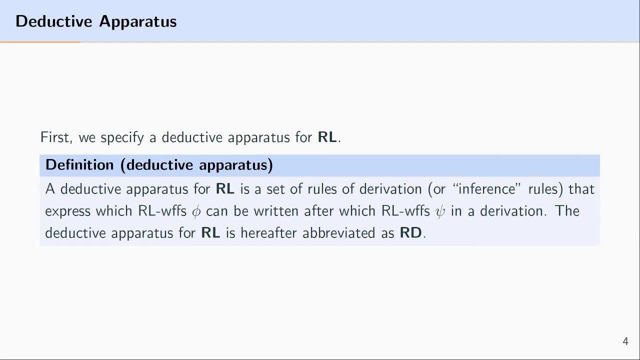 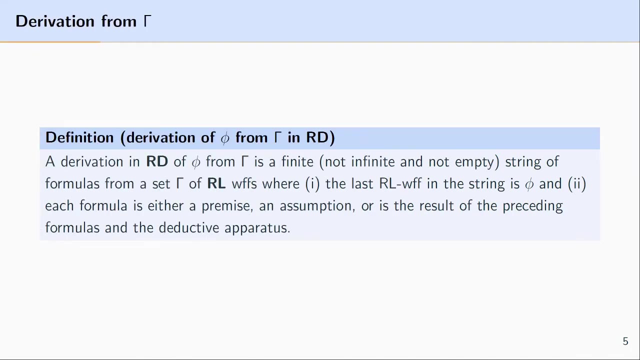 formulas in a derivation. One way of thinking about the deductive apparatus is: it's the set of rules of reason or the permission rules that allow us to move forward in a proof. The notion of a deductive apparatus makes reference to a derivation. I've covered the notion of the 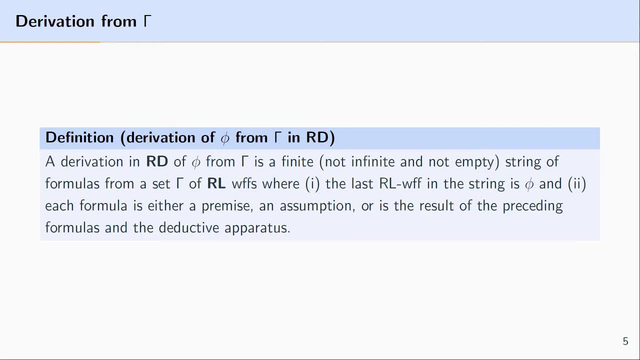 a derivation before, but i just want to briefly cover it again here. all a derivation is is a series, a finite series of well-formed formulas, and we talk about a derivation from a set of formulas, let's say gamma, to a formula, let's say five, and all this is is is a sequence of formulas. 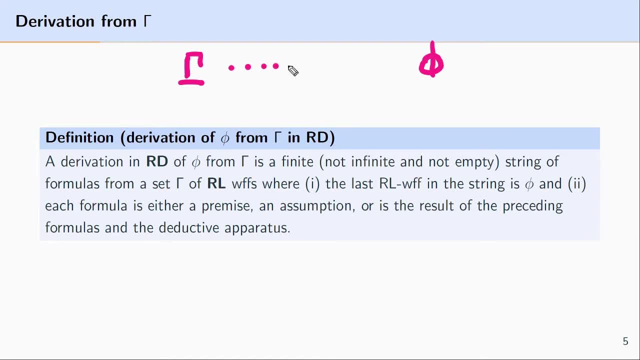 beginning with gamma, and each kind of step in this series is a predicate, logic, well-formed formula, and this series ends in a formula phi. but this series has certain constraints on it. the first constraint is that we begin the series with this set of formulas, gamma, and this gamma might contain. 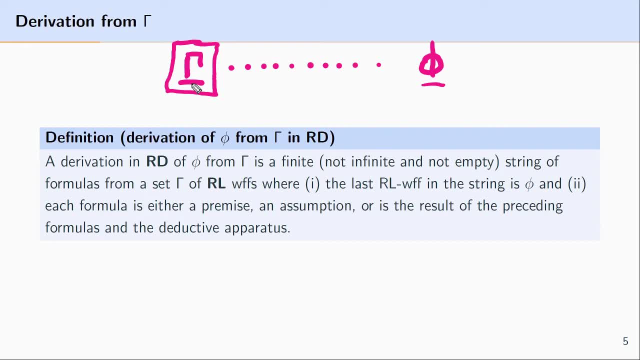 you know, five or six or seven uh formulas. the formulas of gamma are sometimes thought to be, or referred to as, predicate logic formulas, and this series has certain constraints on it. the first premises of the argument. So we're reasoning from these premises that are found in gamma. 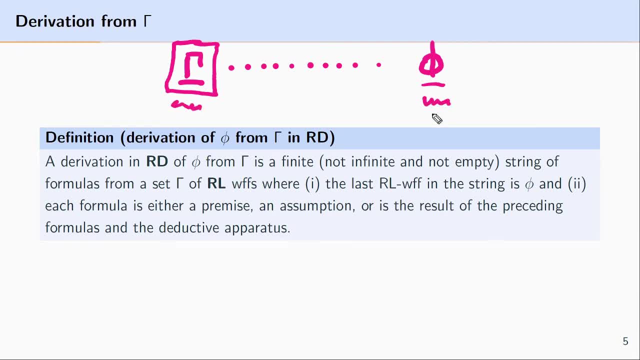 to the formula, the conclusion, which is phi. So a derivation: it begins with gamma and terminates with phi. The final constraint on this series is that each one of these well-formed formulas between gamma and phi is either a premise, an assumption, or is the result of. 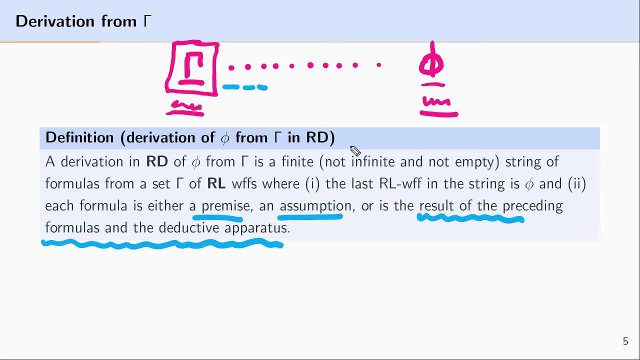 preceding formulas and the deductive apparatus, That is, each one of these formulas, in the sequence from gamma to phi, is justified by our deductive apparatus. In other words, each of the rules is justified by one of our derivation or proof rules. or you can think: 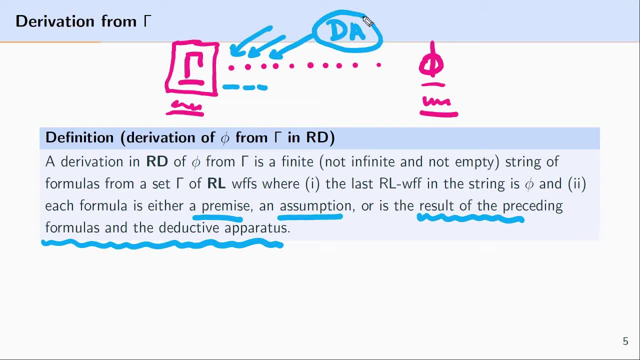 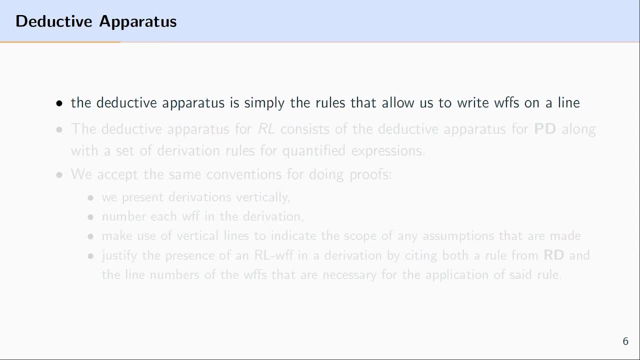 simply the rules that allow us to write well-formed formulas on a line. The deductive apparatus essentially justifies why the new well-formed formula can be put at the line. it's found at The deductive apparatus, for predicate logic consists of the deductive apparatus. 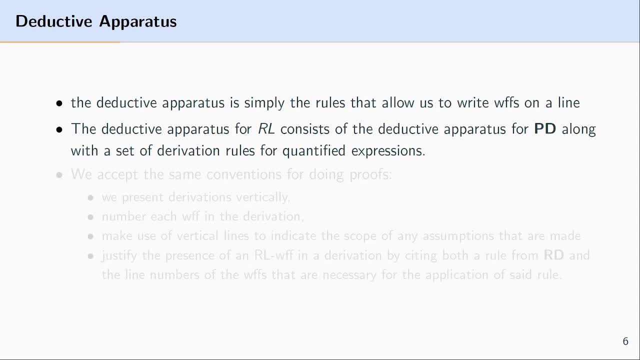 for propositional logic along with the new derivation rules for quantified expressions that we'll develop in future videos. That is, we take all of the rules from propositional logic and we bring them in or import them into the formula, And we take all of the rules. 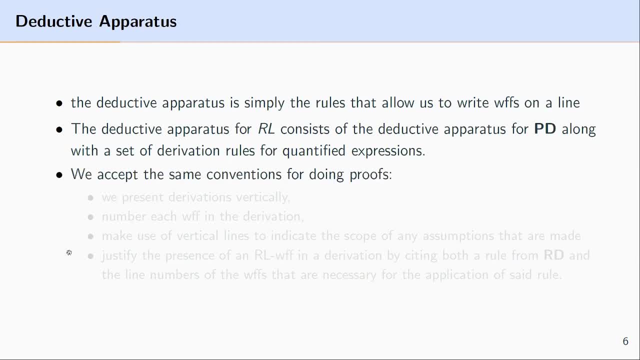 from propositional logic and we bring them in or import them into our rule set for predicate logic. The last thing with respect to this we'll just kind of note about the deductive apparatus is we adopt a lot of the same conventions for displaying proofs, So we'll display the 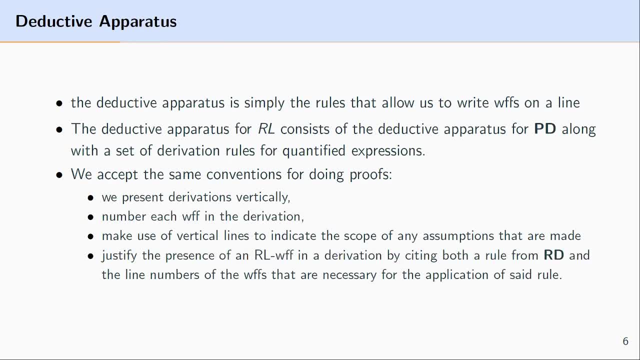 proofs vertically. So rather than simply writing each of the formulas out one right after another in a horizontal row, we'll display them vertically. We'll number each well-formed formula so we can refer back to it. We'll make use of vertical lines as well as indentation to indicate the 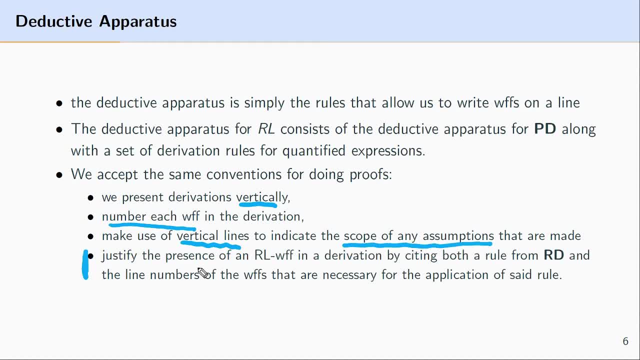 scope of assumptions. We'll also explicitly indicate when we make use of a particular rule from the deductive apparatus, In other words, at each line in the proof. we'll develop some conventions for saying that this line in the proof is here because of the first line and the second.